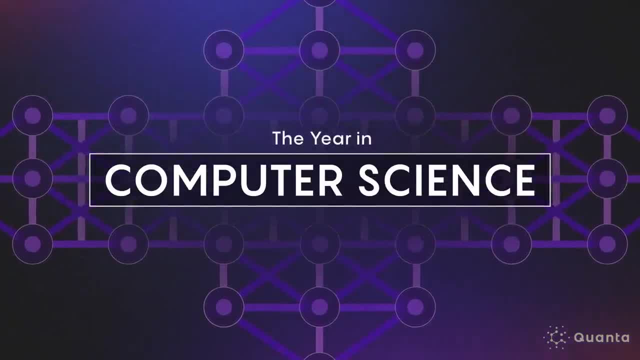 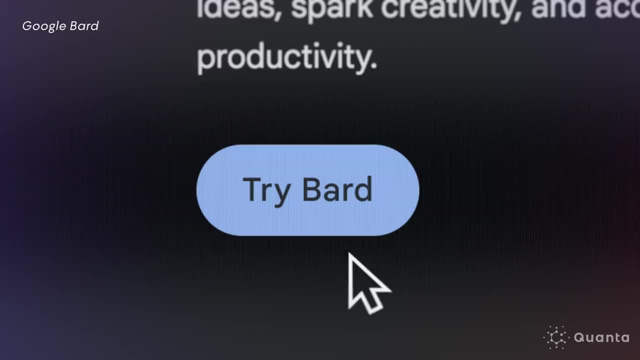 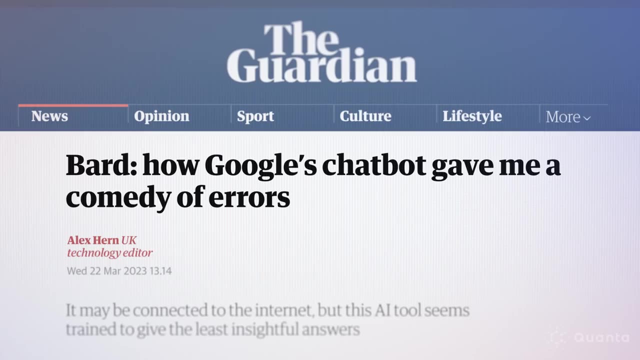 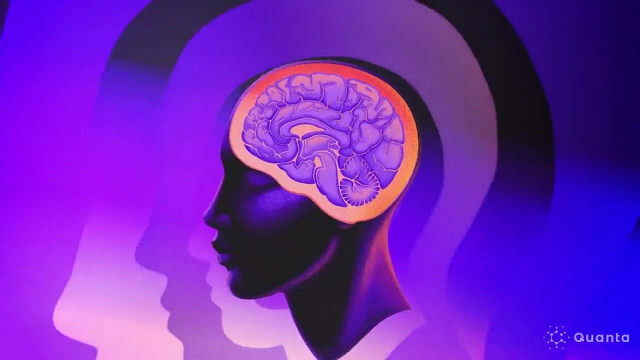 From chat, GPT to DALI. it might seem like the pace of progress in artificial intelligence is unstoppable, But the artificial neural networks that underpin these programs are coming up against some major limitations. For one, they have a hard time reasoning. Human brains are able to reason by. 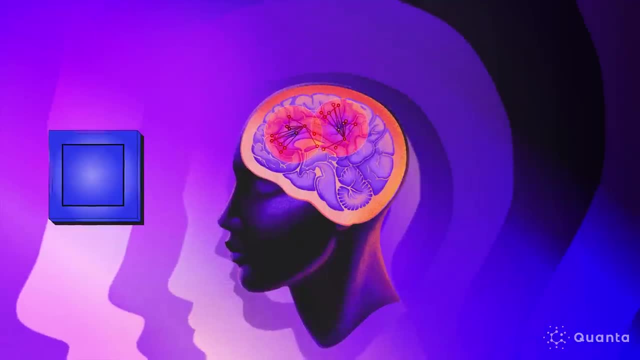 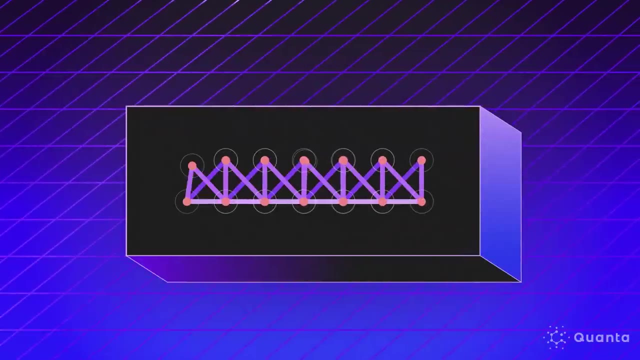 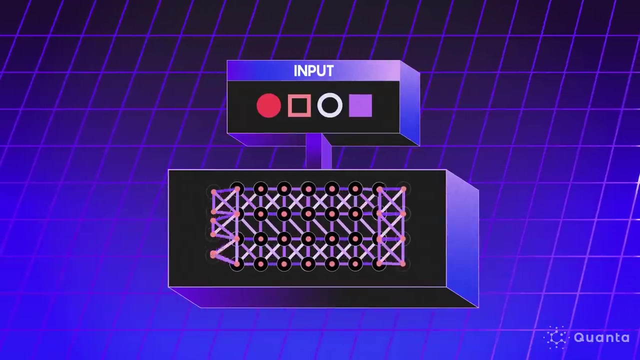 analogy. When we see something new, we don't have to grow new neurons. We can generalize new concepts from existing knowledge, But artificial neural networks struggle to reason by analogy. in this way, When confronting new information, they often require more artificial nodes to scale up their 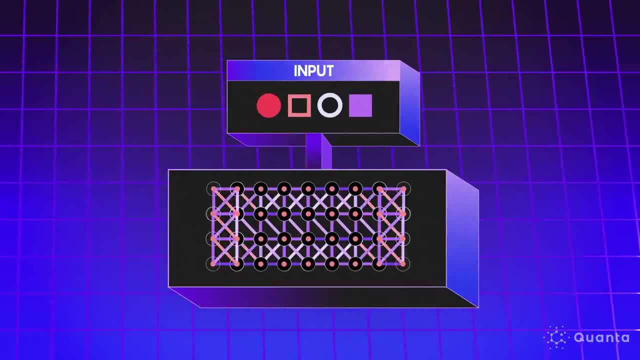 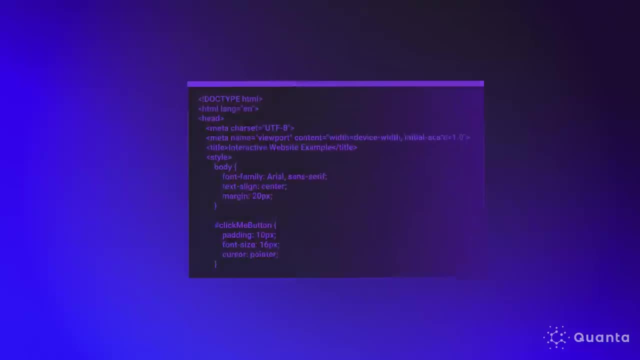 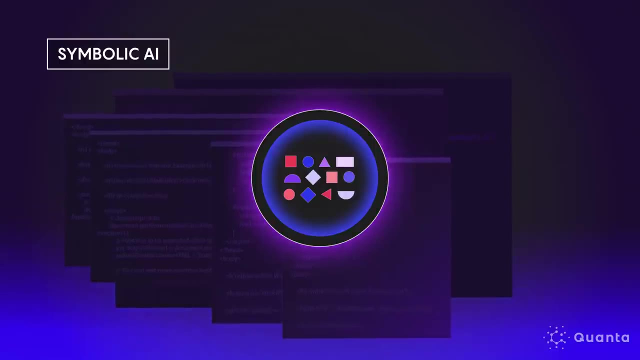 statistical abilities, which enables them to learn new concepts. This approach is called statistical AI. Statistical AI is at the heart of deep neural networks, But there is another competing approach, known as symbolic AI, which uses logic-based programming and makes use of symbols to represent. 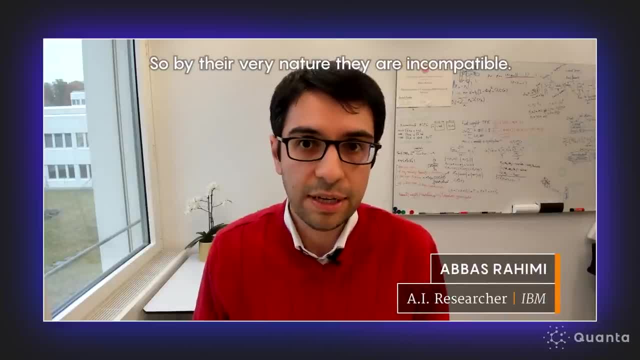 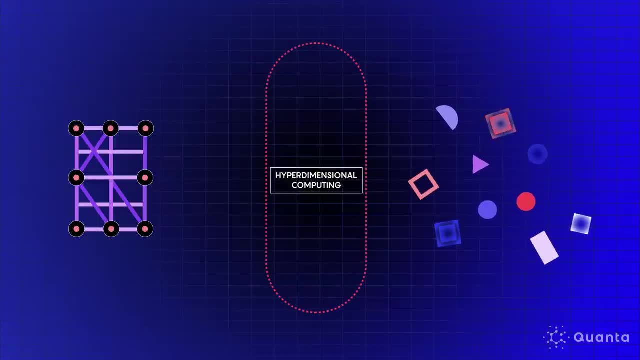 concepts and rules, So by the very nature they are incompatible, And the big challenge is that how we can combine them together to get the best of both worlds. An emerging approach called hyperdimensional computing aims to do just that. It taps into the power of statistical AI, while 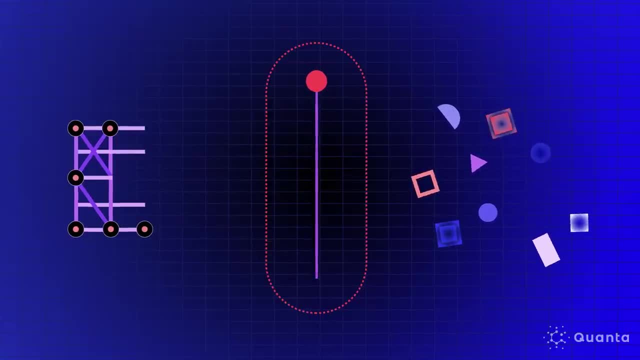 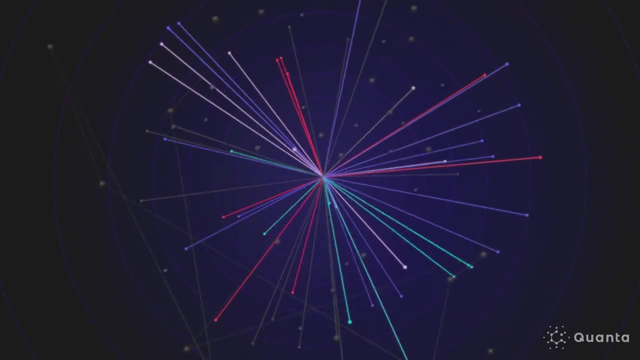 also trying to emulate symbolic computing. It does this by using vectors, ordered lists of numbers that can also represent arrows in space, Depending on where they're pointing. these vectors can represent information in a highly complex, multi-dimensional way. They can embody nuances. 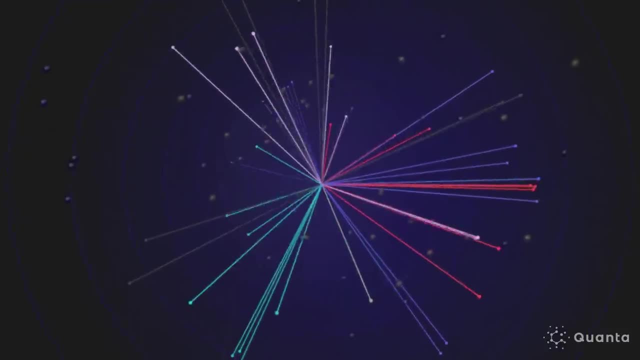 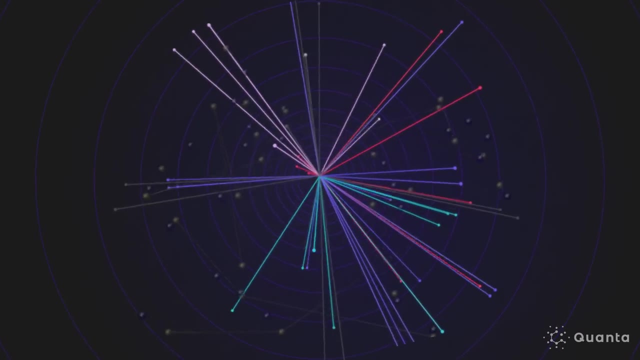 and traits or concepts. just by small changes to their orientation, These vectors can combine to represent new concepts, then be pulled apart again to discern how they were formed. And, crucially, these hyperdimensional vectors can encode information without having to add more nodes. 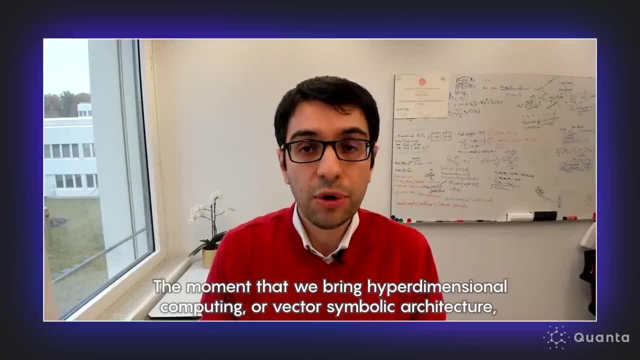 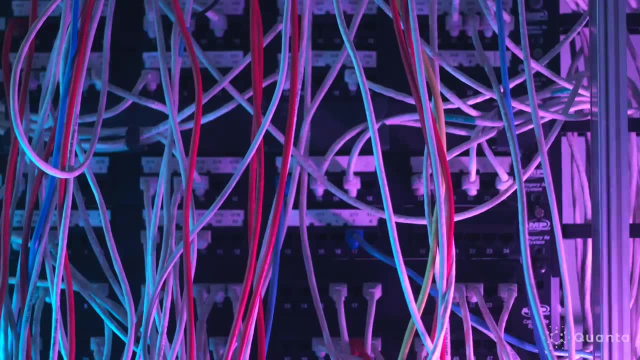 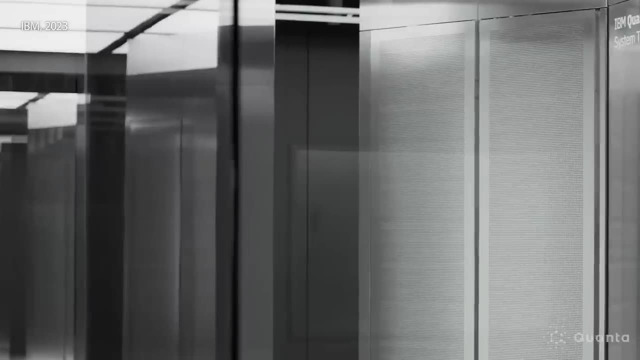 to the network. The moment that we bring hyperdimensional computing or vector specific architectures and marry it with statistical methods, such as deep neural network, we can have certain advantages. In March 2023,, computer scientists at IBM Research in Zurich made a dramatic breakthrough by combining statistical and symbolic methods to solve. 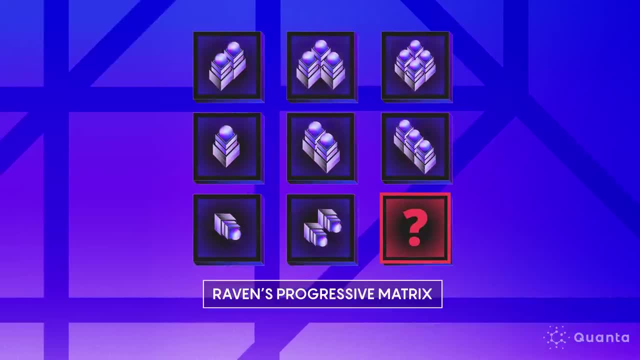 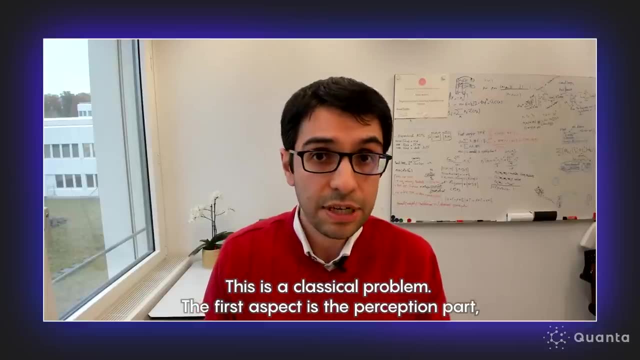 the Raven's Progressive Matrix, a puzzle that asks an AI to predict an image to fill the final square of a three-by-three grid. This is a classical problem. The first aspect is the perception part, where we look at different visual objects and then we have to recognize 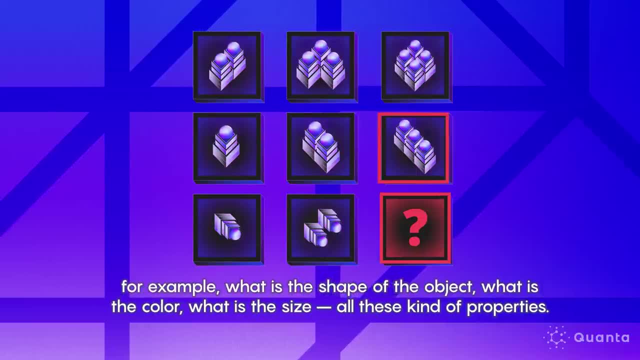 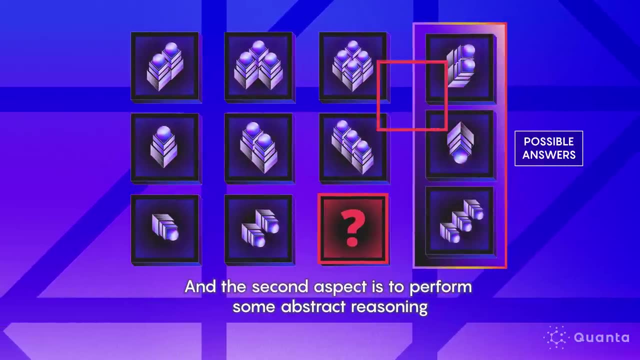 a certain aspect of the object, For example, what is the shape of the object, what is the color, what is the size, all these kind of the properties. And the second aspect is to perform some abstract reasoning on top of these kind of attributes of the objects, to be able to. 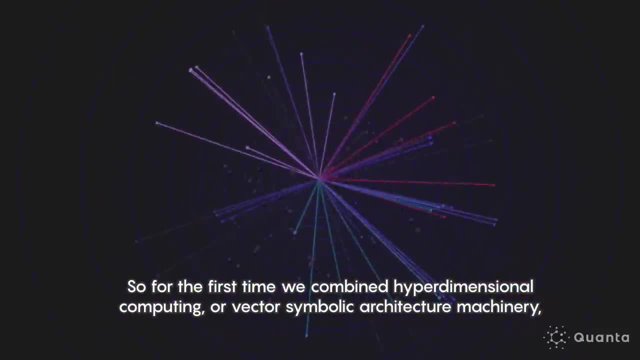 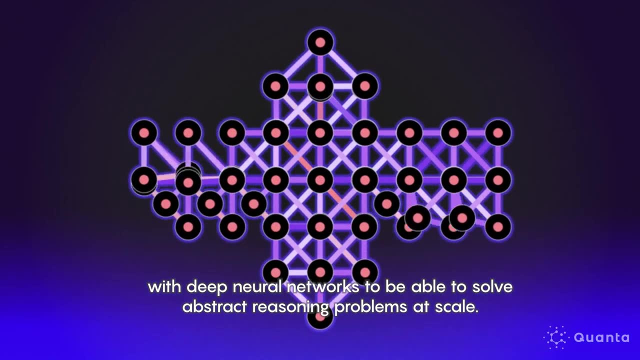 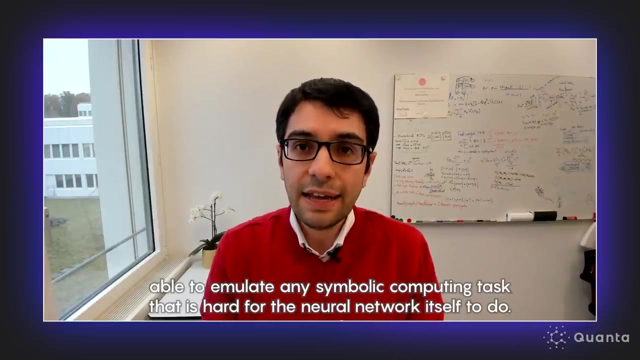 solve a puzzle. So for the first time we combine hyperdimensional computing or vector symbolic architectures, machinery with deep neural networks to be able to solve abstract reasoning problems at a scale. Essentially, we can build inside the neural network a machinery that is able to emulate any symbolic computing task that is hard for. 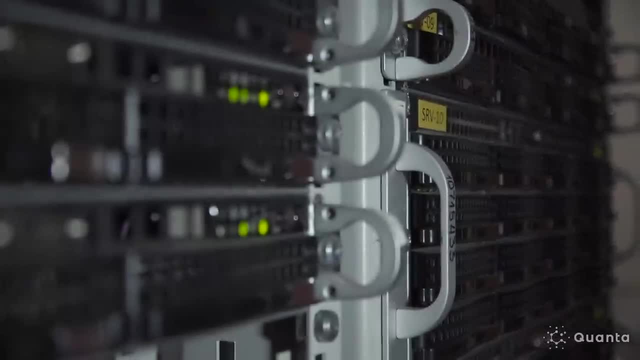 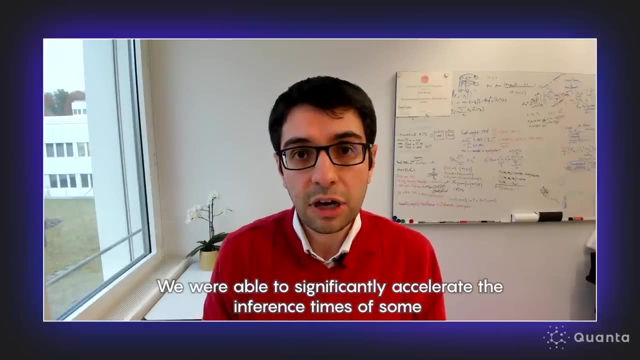 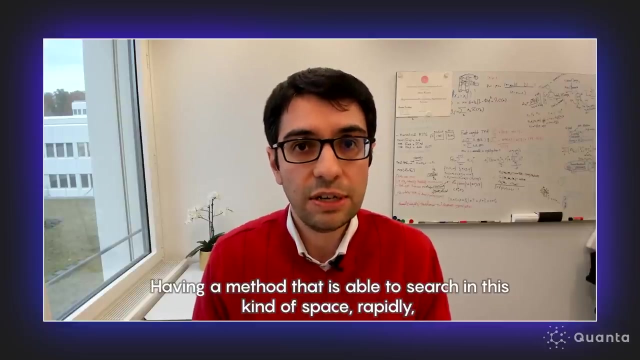 the neural network itself to do. The researchers also broke new ground by solving the problem in record speed. We were able to significantly accelerate the inference times of some of the abstract reasoning tasks by 250 times. Having a method that is able to search in this kind of the space rapidly, it's quite crucial to be able to make them. 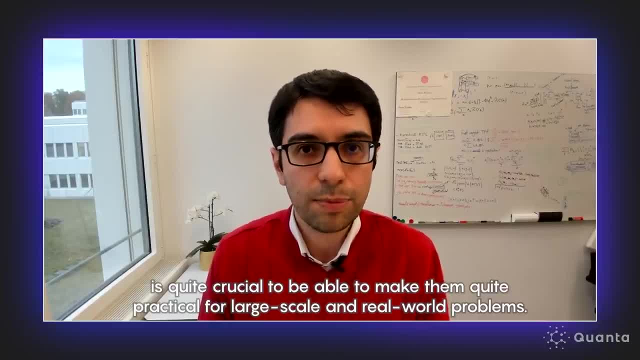 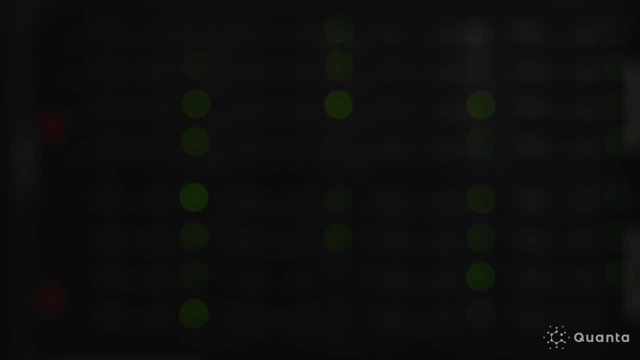 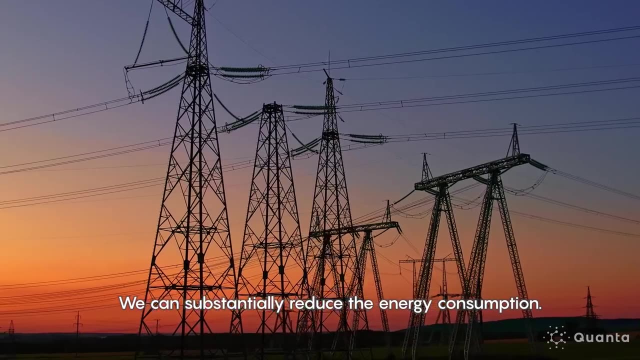 quite practical for larger scale and real-world problems, Although more work is needed. researchers like Rahimi hope that hyperdimensional computing could be faster, more transparent and more energy efficient than current AI platforms. We can substantially reduce the energy consumption We are talking about, you know. 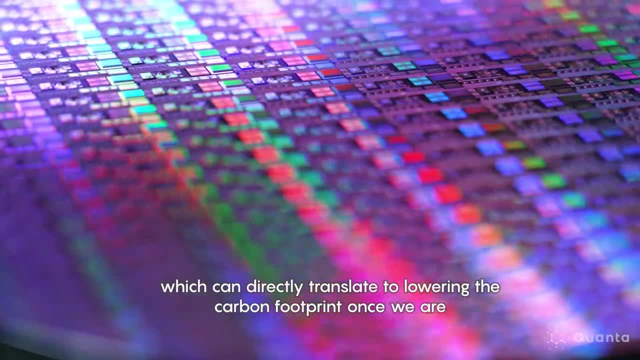 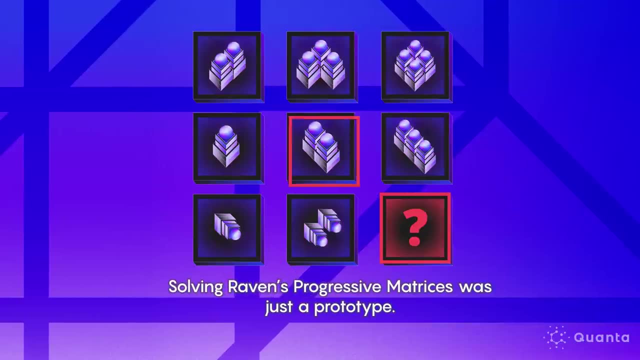 10 times to 100 times lower energy consumption, which can directly transfer to lowering the carbon footprint once we are performing. the inference of this kind of the models Following Raven Progressive Matrices was just a prototype. It was so far amazing, but the fun is just beginning. 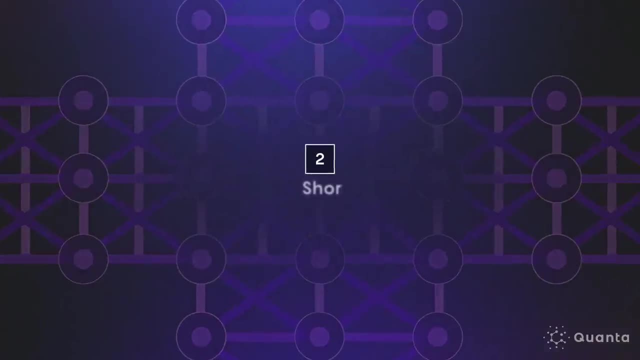 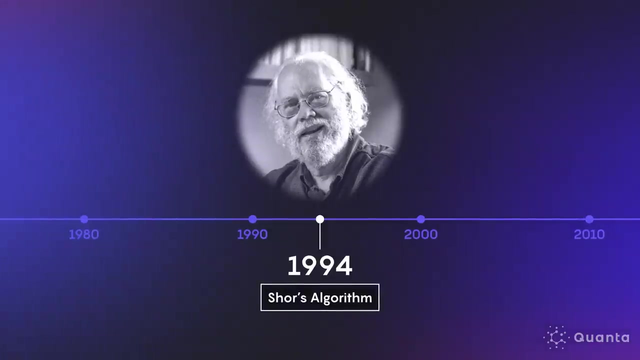 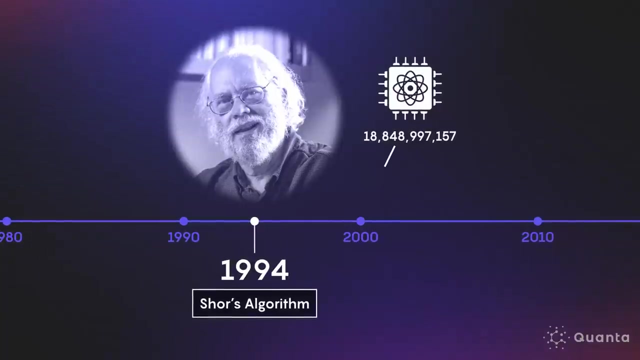 That's the beauty. In the 1990s, mathematician Peter Shor developed an algorithm that threatened to break the internet. He was trying to understand the power of quantum computers and realized that they would be able to rapidly break large numbers into their prime factors. 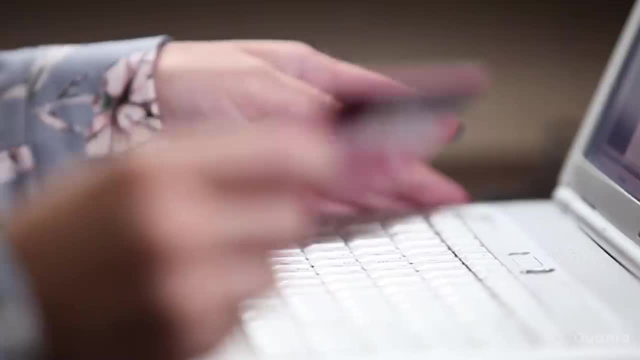 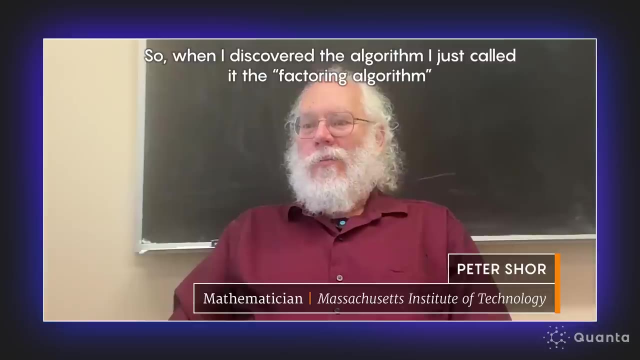 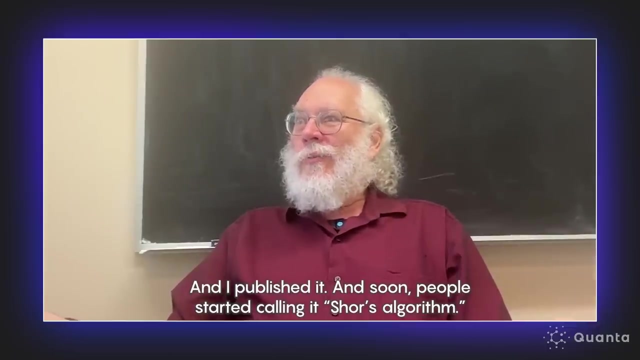 That would undermine one of the central methods of modern cryptography that has safeguarded online privacy for decades. So when I discovered the algorithm, I just called it the factory algorithm or the quantum factory algorithm, and I published it, And soon people started calling it Shor's algorithm. 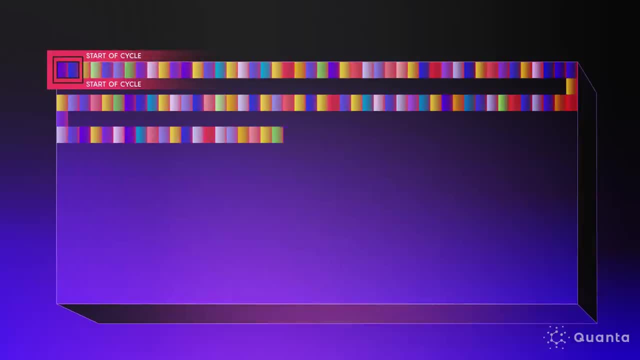 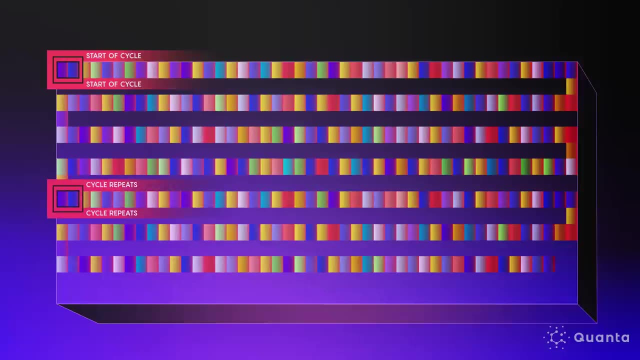 At the heart of Shor's algorithm is the act of repeatedly multiplying one number with itself until the output of a certain function starts repeating The required number of multiplications, called the function's period, can be used to find the prime factors of any large number. 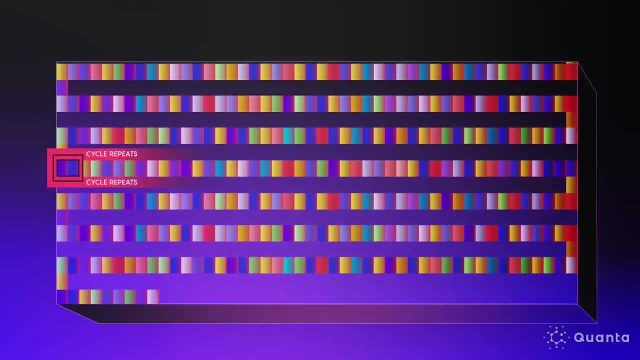 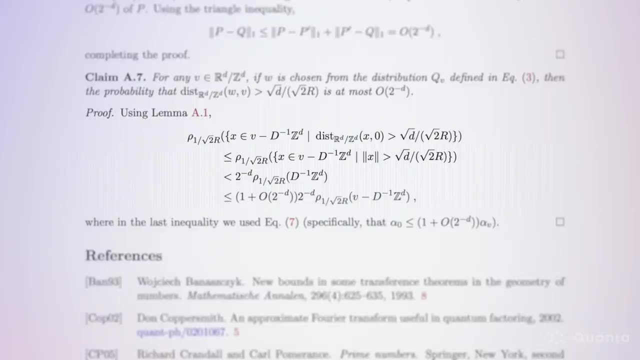 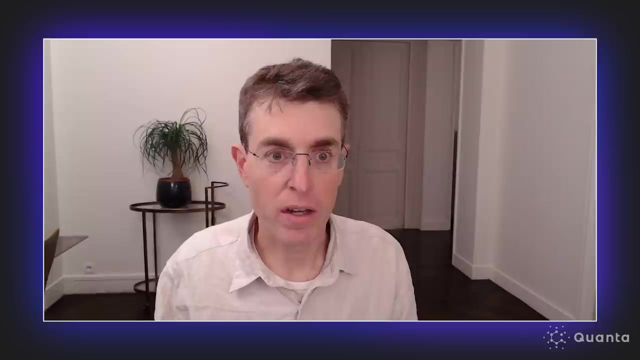 For the last 30 years, this has been the fastest-known algorithm for factoring integers. Then, in August 2023, mathematician Oded Regev published a groundbreaking new paper. Shor's algorithm is great in the sense that it allows quantum computers to factor as integers. 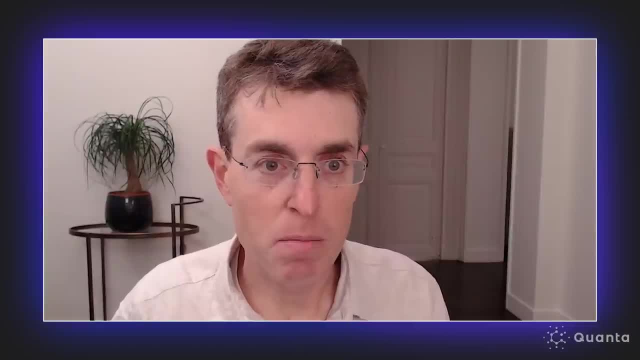 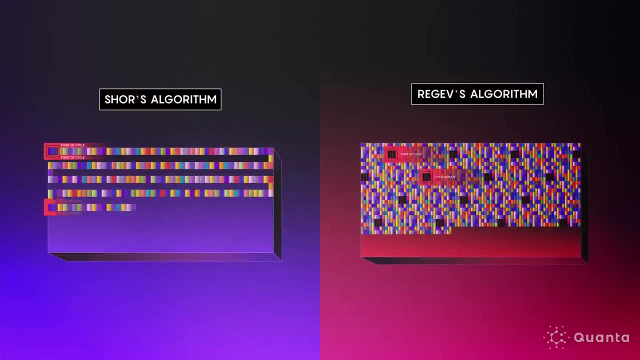 and do it quickly. I was asking myself if it can be made even faster. Regev suspected that he could speed up Shor's algorithm by transforming the periodic function from one number to two, From one dimension to multiple dimensions. That meant including more numbers. 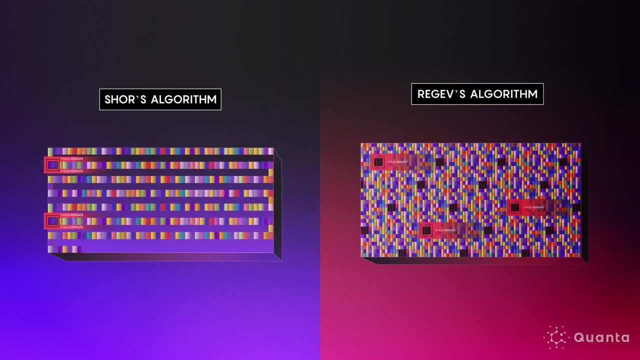 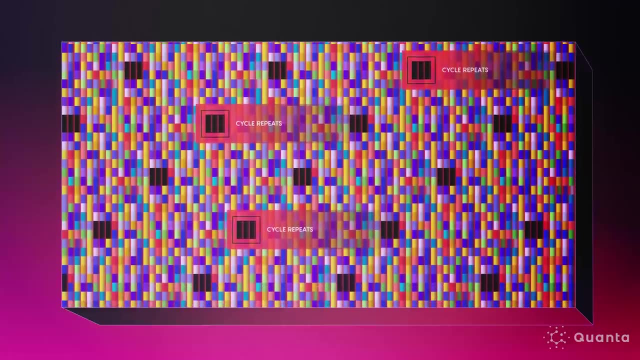 multiplying each with itself many times over to find the period of repetition in the outputs. In doing so, Regev established an improved method to factor integers faster and more efficiently. Shor's algorithm is about finding how long you have to walk on the line. 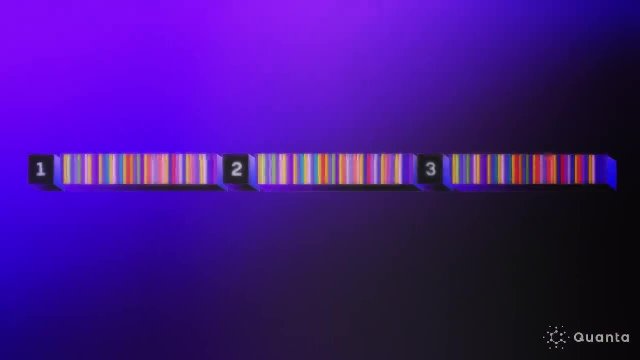 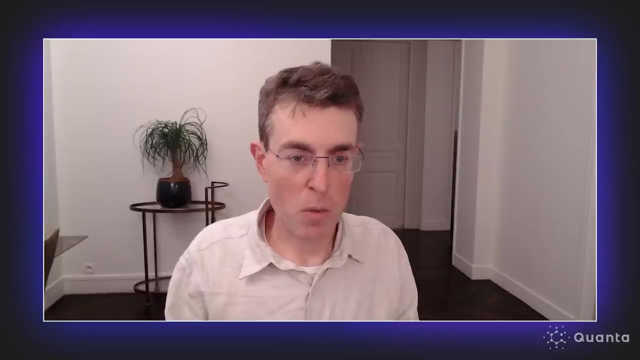 to get back to where you started. In the new algorithm, we no longer walk on a line, We walk on a plane or even three-dimensional space or more. The idea is that you can walk both right-left but also top-down on the plane. 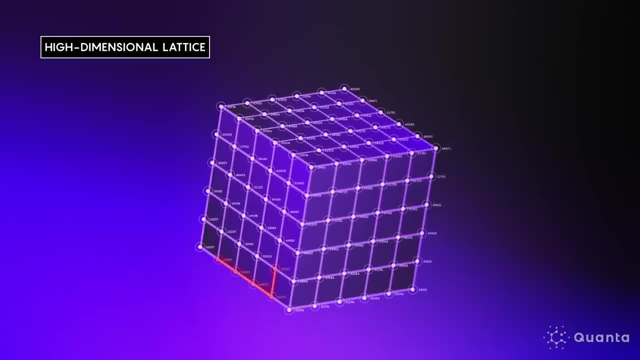 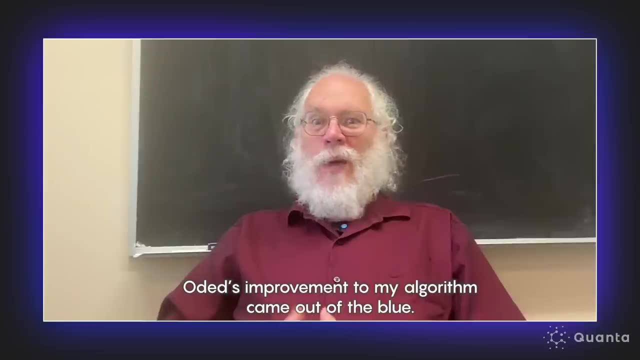 So it could be. for instance, if you walk four steps to the right and five steps up, you'll be back to where you started from. Oded's improvement to my algorithm came out of the blue. There wasn't any work leading up to it. 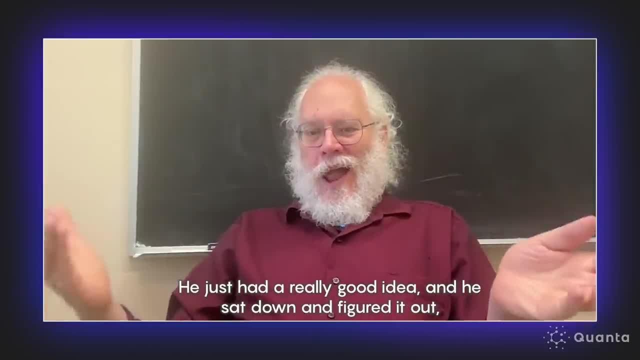 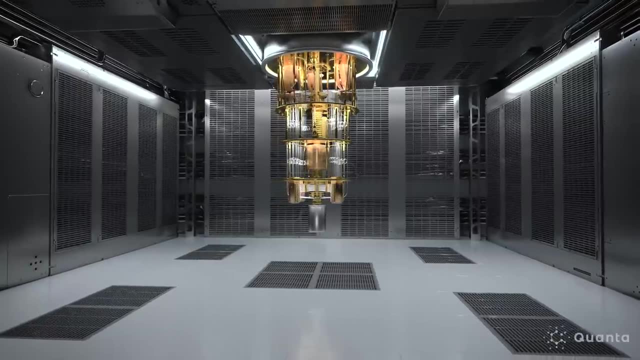 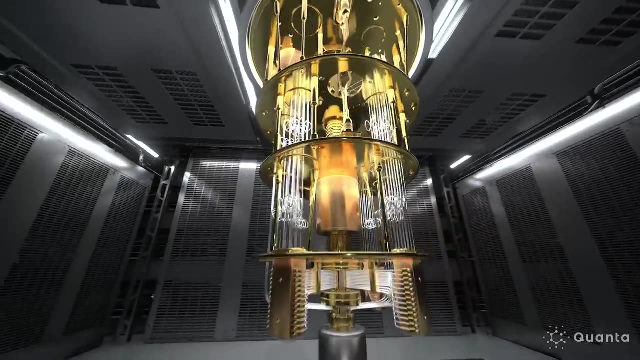 He just had a really good idea and he sat down, figured it out and published a paper. Like Shor's algorithm, Regev's new algorithm remains theoretical in nature, speaking to a potential future when quantum computing becomes more practical. 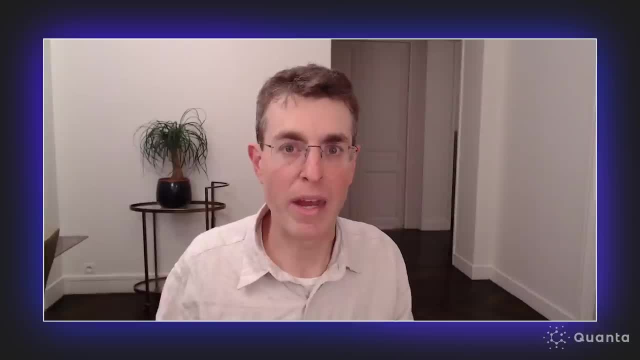 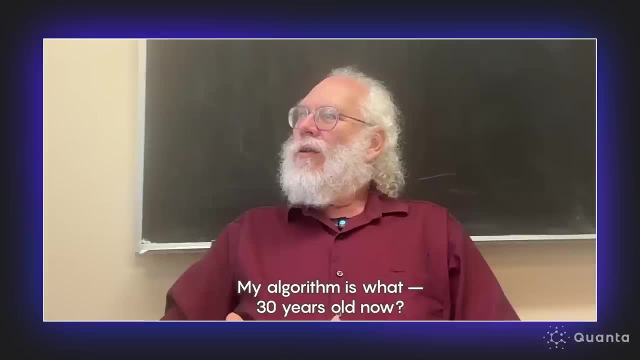 I would be happy if it turns out that this new algorithm is more practical. It has some of the components that could make it more practical, but it's not clear yet if it's really there. My algorithm is what? 30 years old now. 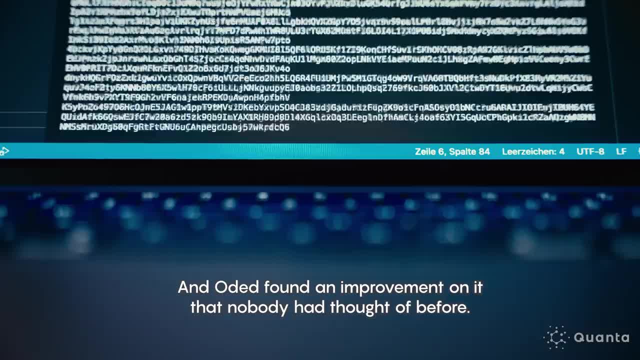 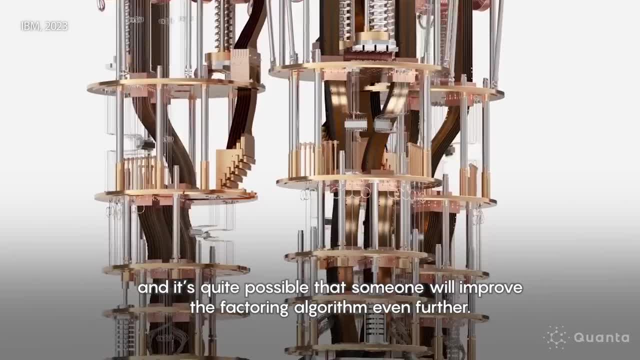 And Oded found an improvement on it that nobody had thought of before. I wouldn't be surprised if people came up with more, in a way, more practical algorithms. I know they have quantum algorithms and it's quite possible that someone will improve. 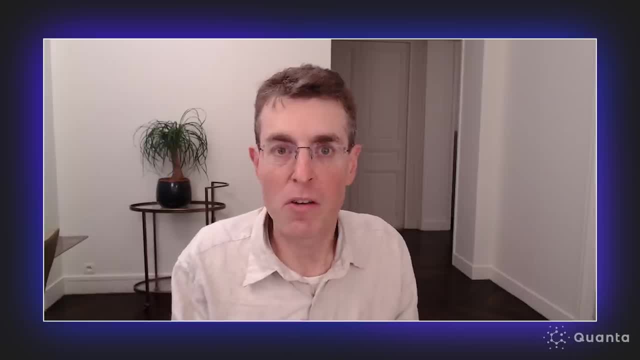 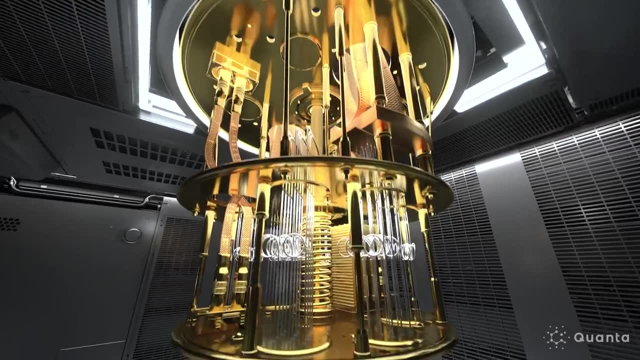 factoring algorithm even further. We already knew how to factor as integers using Shor's algorithm, So this new algorithm is kind of just a speed up. What I would really like to know is if quantum computers can do things that we just didn't know how to do. 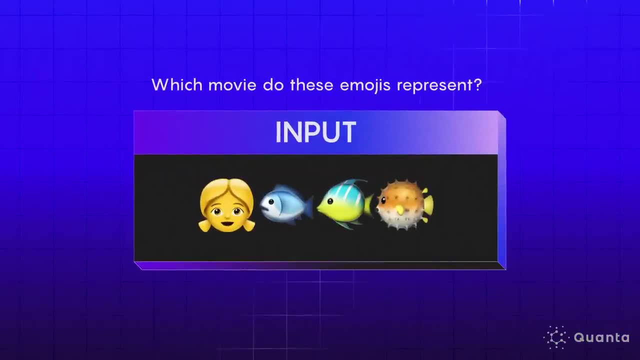 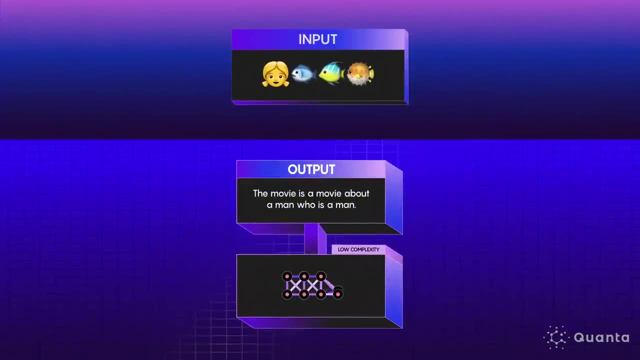 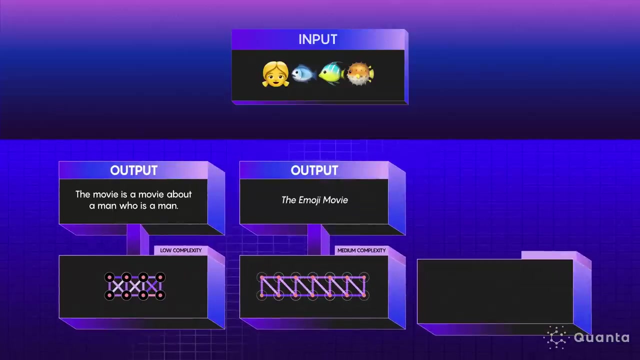 Which movie do these emojis represent? When researchers asked three different large language models, they got very different answers. The simplest AI struggled to come up with a coherent answer. A somewhat more complex model spit out something reasonable, but still wrong. But the most complex system nailed it in just one try. 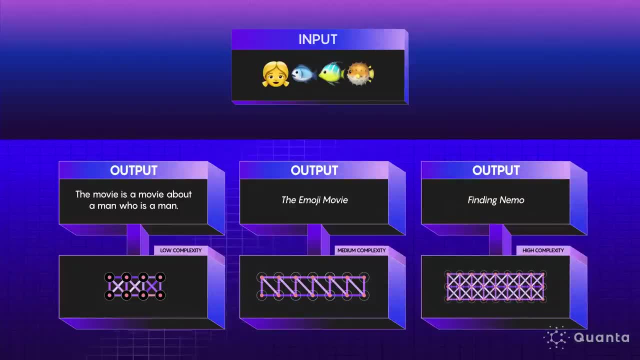 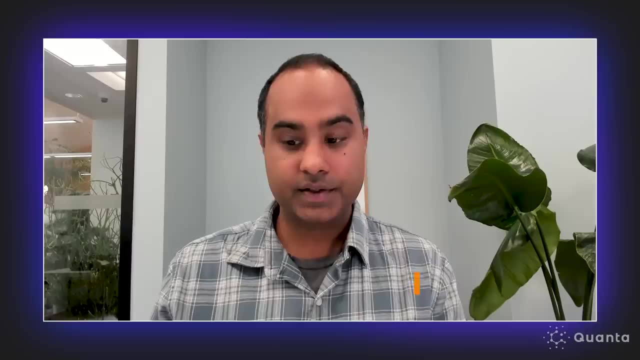 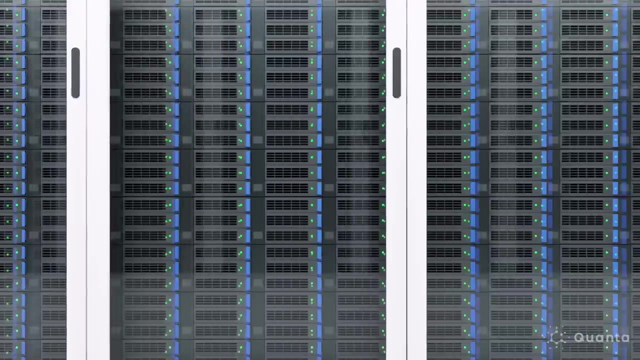 This impressive result can be explained by a range of exciting new abilities. AI researchers are calling emergent behaviors Something that is not present in a small language model that becomes present in a larger model. it can be said to have emerged. We don't think that it'll be there. 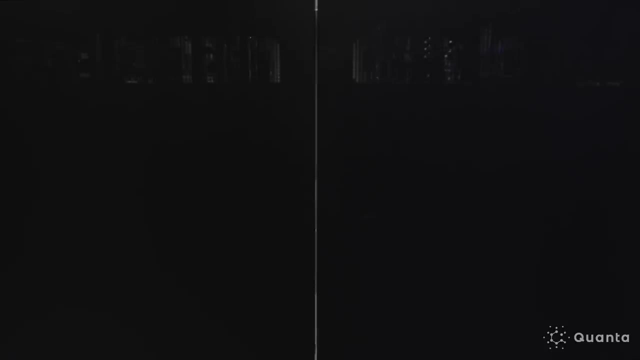 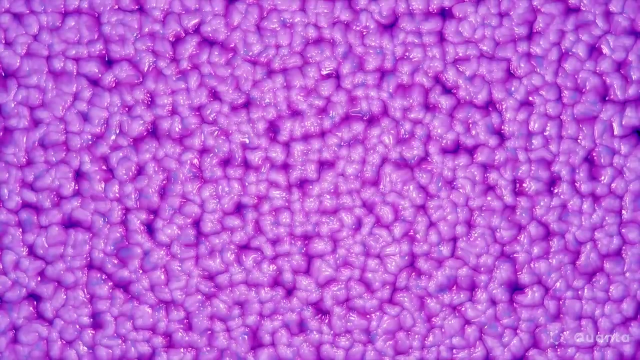 and then we scale it up and all of a sudden this phenomenon is already there, And so it's not necessarily a predictable phenomenon. Emergence happens when a system behaves in ways its individual units don't on their own. This phenomenon can be seen across nature. 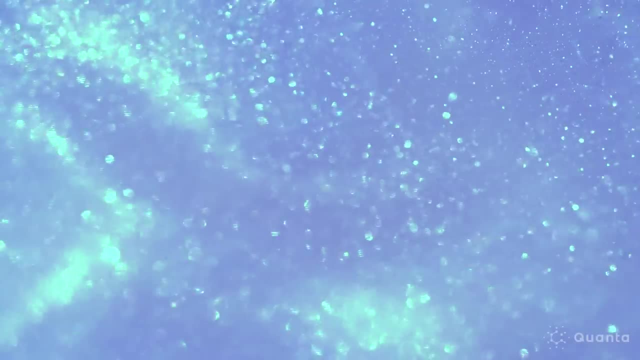 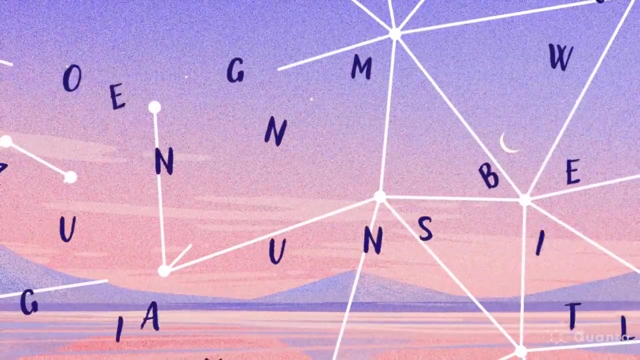 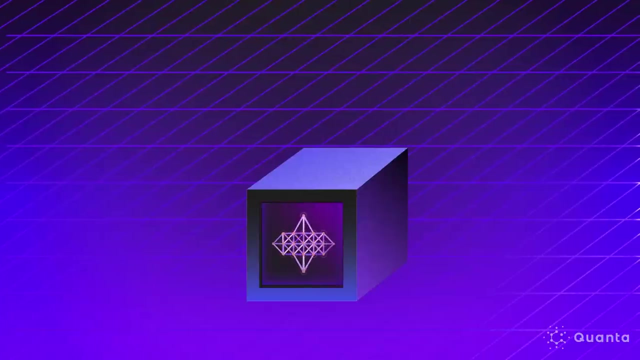 such as when lifeless atoms give rise to living cells, water molecules create waves and starlings swarm and swoop as one. Researchers are seeing that if enough digital nodes combine in large language models, surprising new behaviors can emerge. These behaviors are a distinct departure. 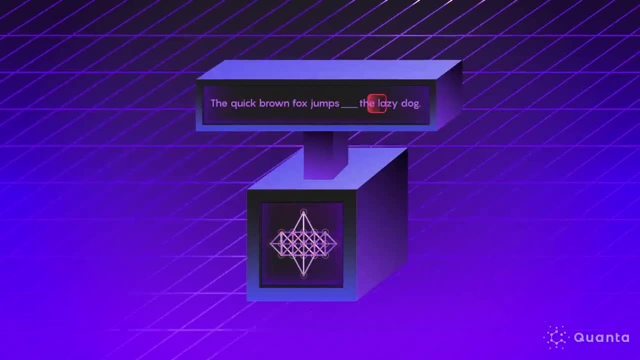 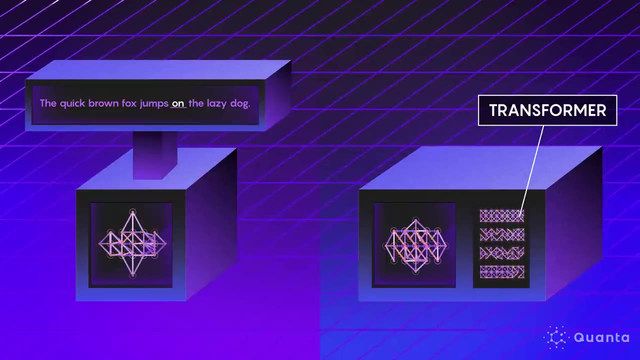 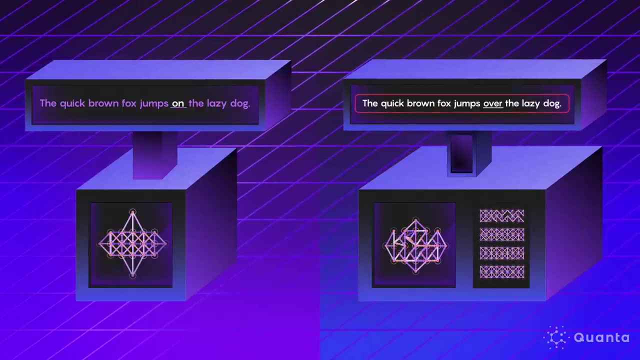 from older neural networks which process language word by painstaking word. In 2017, a key piece of code known as a transformer was introduced to LLMs, enabling neural networks to analyze words in parallel. Now, LLMs can process strings of text in an instant. 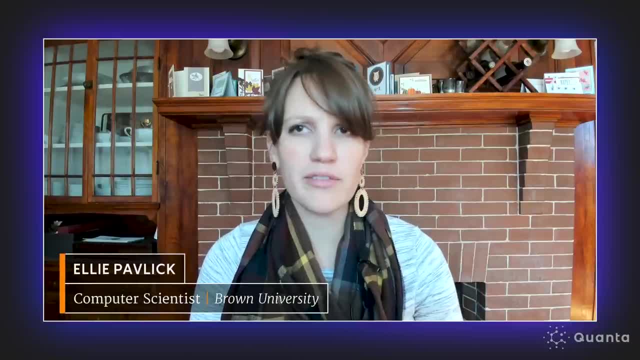 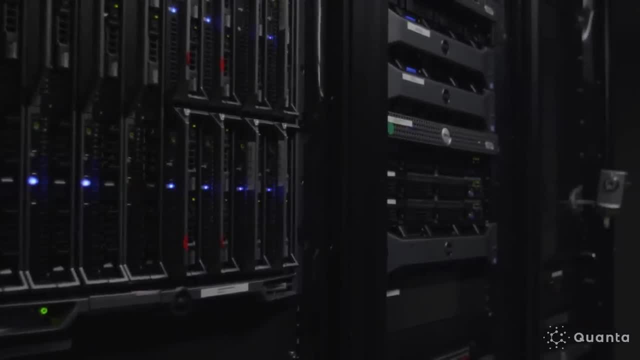 The models we were training before seemed to be, you know, seemed to struggle with a lot of kind of more abstract tasks, more generalization, And what we've seen since transformers is that if we train much larger models, they're better at those tasks.